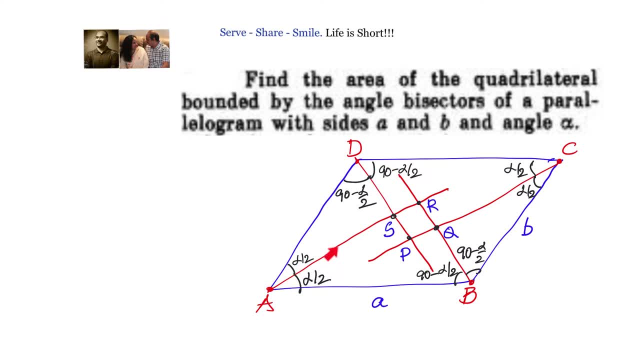 quadrilateral, PQRS, which is formed by joining the angular bisectors of the parallelogram. So we have AR, then BR, CP, DP. These are all angle bisectors. When they meet with each other, the area bounded is PQRS area, That is, now we have to find out the area of that particular quadrilateral. So to 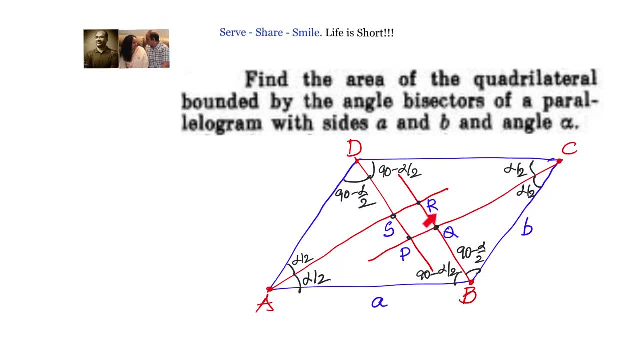 proceed with the problem. let us understand what will be PQRS, What type of quadrilateral PQRS will be. So for that they have given us extra information. They said that sides are A and B and the angle of parallelogram is alpha, Since it is an angular bisector. now alpha is divided into alpha. 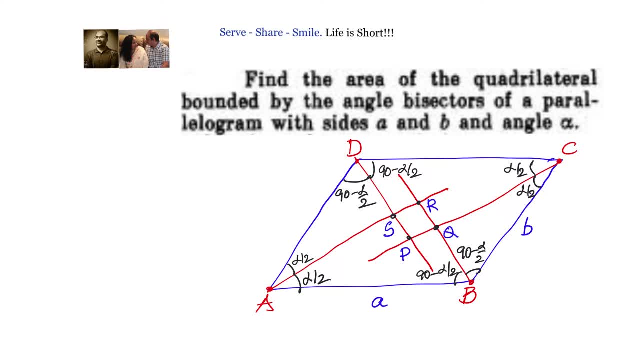 by 2, alpha by 2, and when we go to angle at D, we know that A plus D is 180 degrees because we have entry in a parallelogram. So and that is divided into two equal parts. So we have 90 minus alpha by 2. 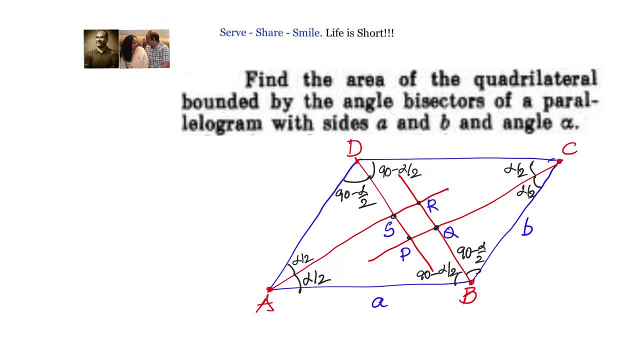 90 minus alpha by 2.. Similarly at B and C also. Now, when we do anglesome property on the triangle ASD and BQC and ARB and DPC, we can see very clearly that each of this angle is equal to 90 degrees. So what we have now is a rectangle. So PQRS is a rectangle. So let us go ahead and put. 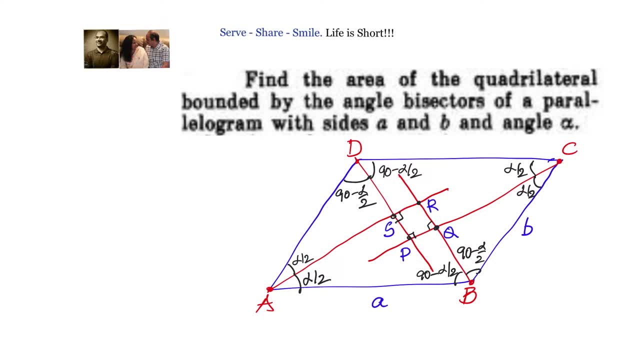 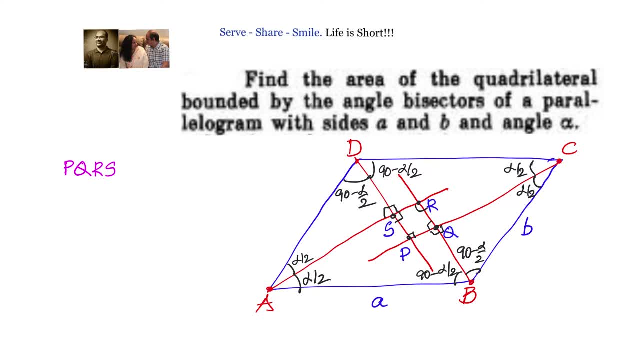 So we can say that PQRS is a rectangle. So we can say that PQRS is a rectangle Because all the angles are equal to 90 degrees. Now, once we know PQRS is a rectangle, what is the area of a rectangle? length into breadth? 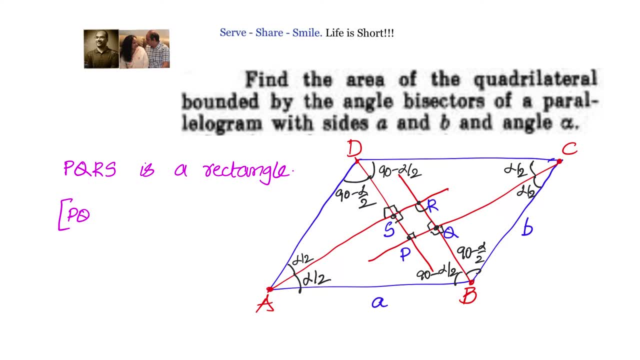 So can I say that area of PQRS is equal to RS into R cube. So can I say that area of PQRS is equal to RS into R cube. So can I say that area of PQRS is equal to RS into R cube. 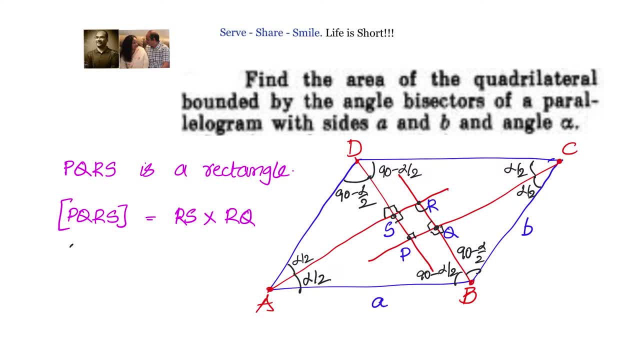 Now, what is RS? RS is nothing but equals to AR minus AS. Multiply that with RQ, which is BR minus BQ. Now let us see what is AR and what is AS, If you take this triangle AB and BR and BR. 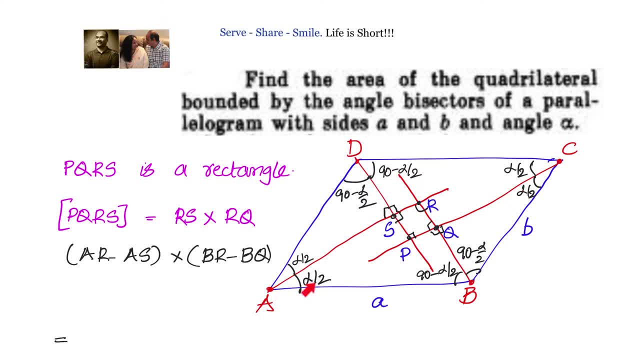 you can look from here. What we want to find out is AR. AR is adjacent side, So cos alpha by 2 will give you AR divided by A. Or can I say AR equals to A into cos alpha by 2?? So we can say A into cos alpha by 2, minus AS. 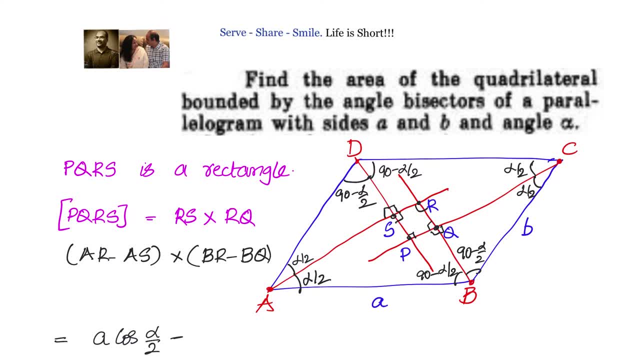 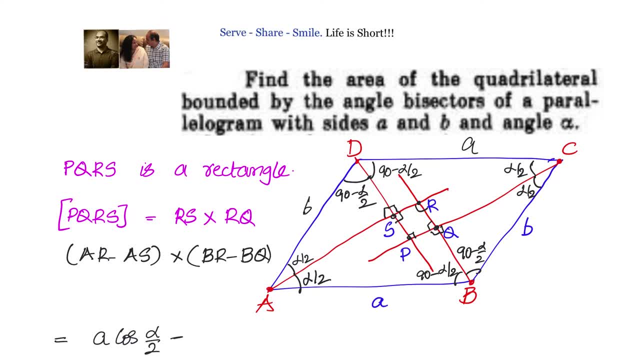 and that very thing is B into cos, alpha by 2.. Now we can check that from the triangle ASD, because alpha by 2, multiply that with BR, Then we can see that BR from triangle ARB is actually A sin: alpha by 2.. 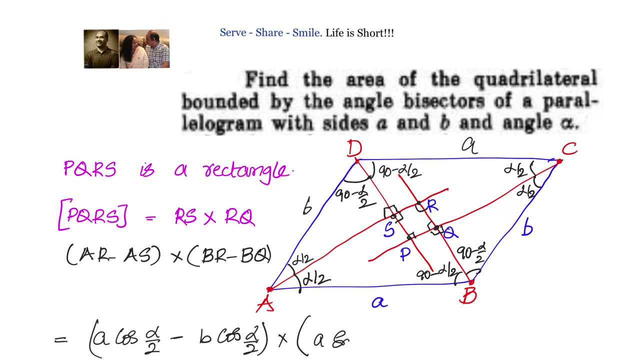 We can even add this to the triangle- can also be A sin alpha by 2.. Then we can see that BR from triangle ARB is actually A sin alpha by 2.. And from triangle BQ we can use BQ into B2, into A你要. 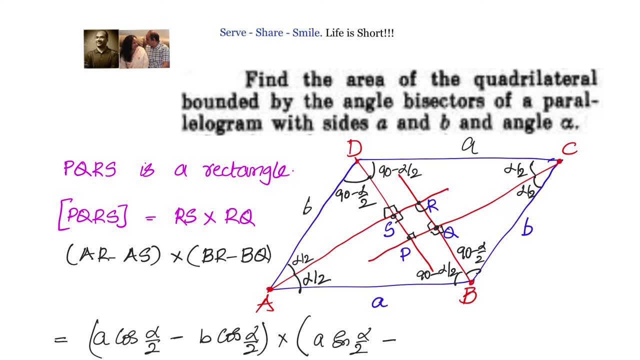 triangle bqc, we can see that bq equals to b sine alpha by 2.. Now let us simplify this. what we have is a minus b whole square into sine alpha by 2, cos alpha by 2. we can leave it like that, or we can write it as half into a minus b whole square into sine alpha, because we know that. 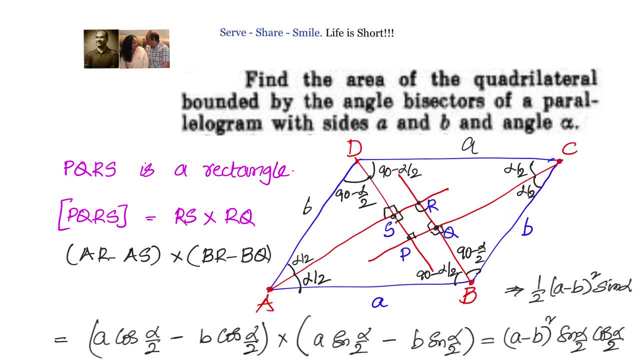 sine alpha equals to 2 sine alpha by 2 cos alpha by 2.. So let us have a recap of this problem. we have been asked to find out the area of the quadrilateral which is bounded by the angular bisectors of the parallelogram. So now the angular bisectors are drawn, then we found out that